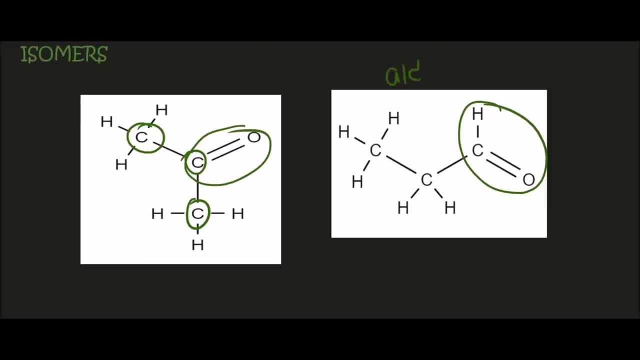 So it's at the very end of the chain. Okay, so this is your aldehyde and then this is your ketone. Now, the general formula for the ketone was: Let's see if that makes sense. We've got one, two, three carbons. 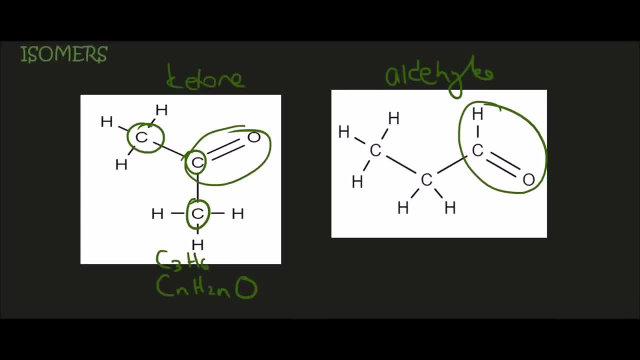 Okay, so that's C3.. Then we've got six hydrogens, and then we have an oxygen. Let's look at the aldehyde. Well, we said that the aldehyde is also going to be CnH2n, and then O. 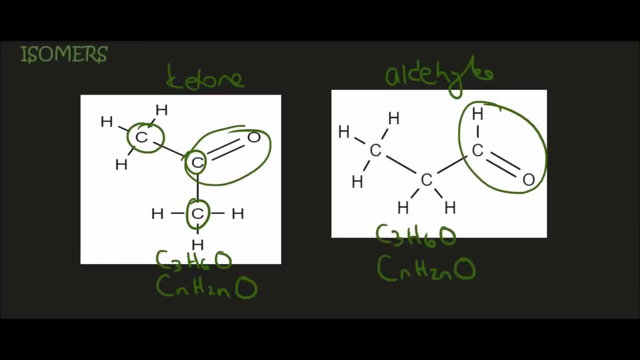 Because we have Here, we have C3H6 and O. So look at this, guys: Both of these molecules, which are completely different because the one's an aldehyde, the one's a ketone, they both have the same molecular formula. 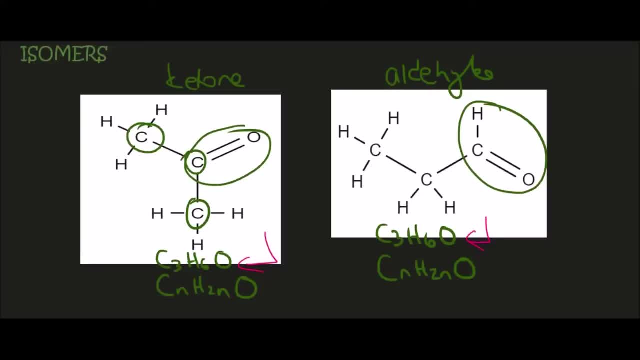 So if you had to read this molecule in a textbook, you would think they're the same thing, And so this is where I'm going to redo the definition of isomers. So let's bring that up once more. So we said that they are molecules. 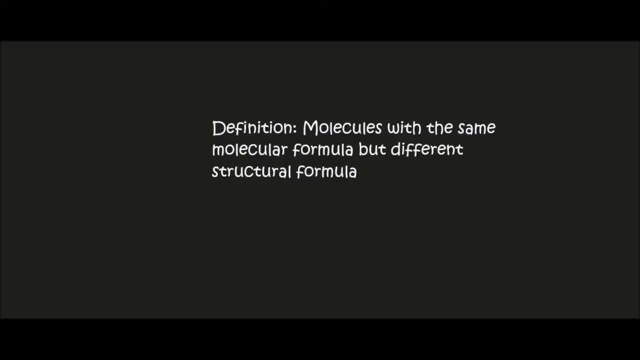 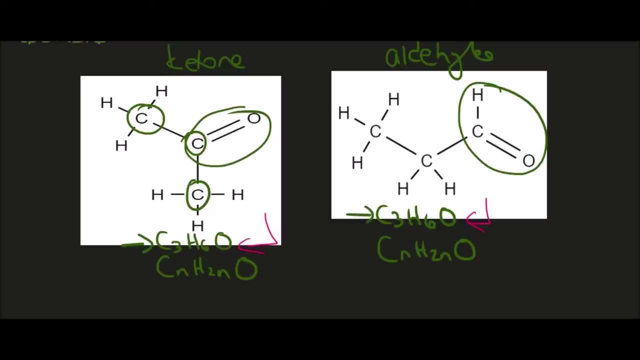 So remember we said that they are molecules with the same molecular formula. So this part here that's the molecular formula. If I use it in terms of N, like variables, then that's called the general formula. But the actual one that I've got here that's called the molecular formula. 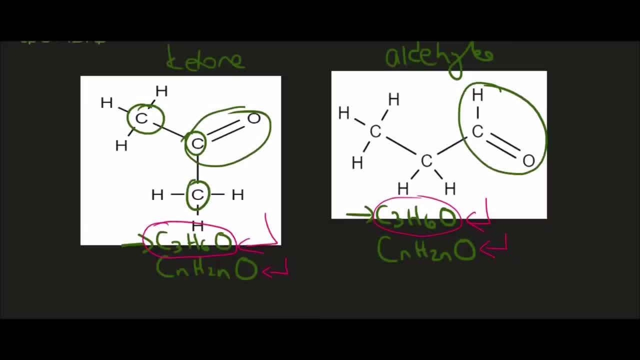 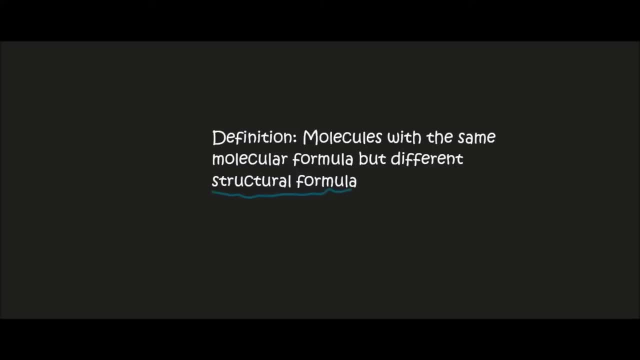 Okay, so both of these have the same molecular formula, And then carrying on, but with different structural formula. What they mean by structural formula is the way that it looks when you draw it, The structure, And so of course we can see that the structure's different. 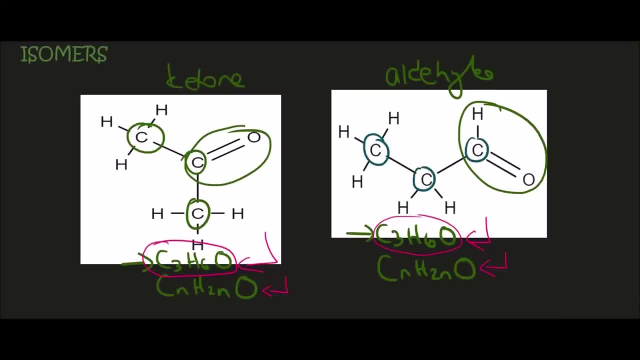 The one on the right has three carbons and then the double bond oxygen at the end. The one on the left has three carbons but the double bond oxygen in the middle. So they are structurally different. So that is what isomers are. 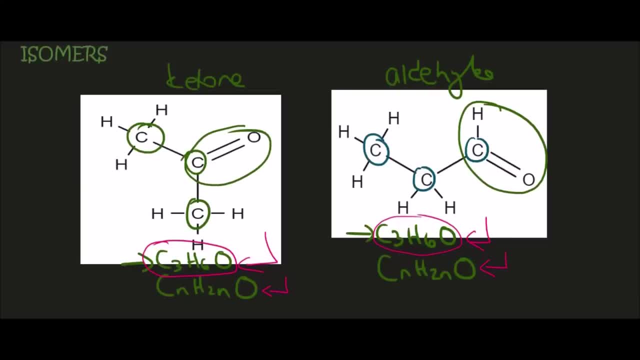 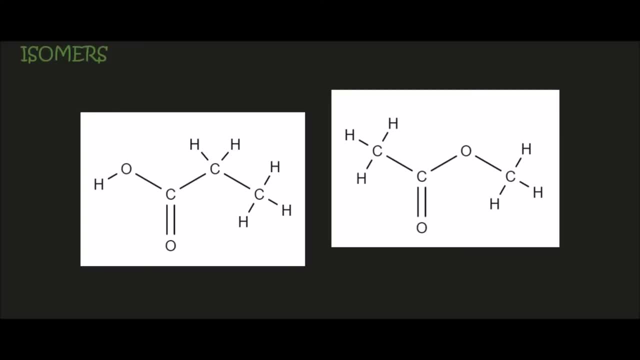 We found isomers between esters and carboxylic acids as well, So let's examine those quickly. So here, if we look at this one, if we look at the left, well, is that the ester or is that the carboxylic acid? 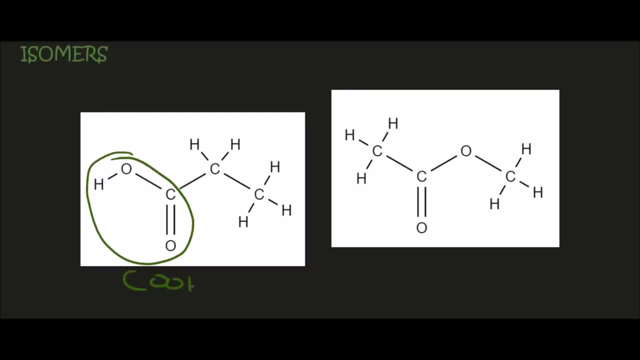 Well, here it's got that Cu part, you know the C-O-O-H. Now that's a carboxylic acid, So I'm just going to say carboxylic, Then you've got a random oxygen in the main chain. 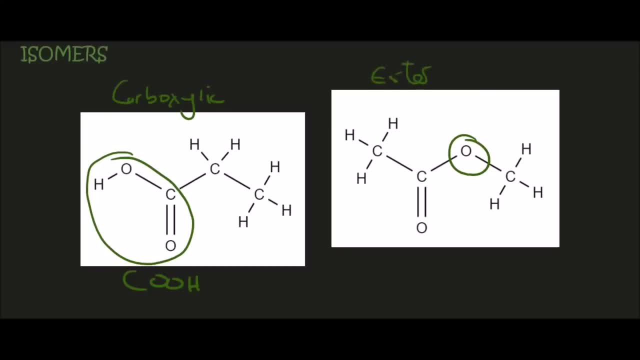 And so that's your ester. Let's quickly look at the molecular formula. Well, the first one has one, two, three carbons, I'm going to say C3. Hydrogens will be one, two, three, four, five, six. 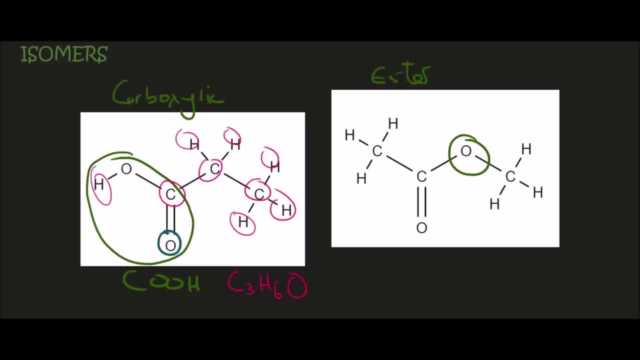 And then oxygens will be one and two, And so we have C3H6O2.. That's the molecular formula. If we look at the one on the right, well, that's got one, two, three carbons, So that's C3.. 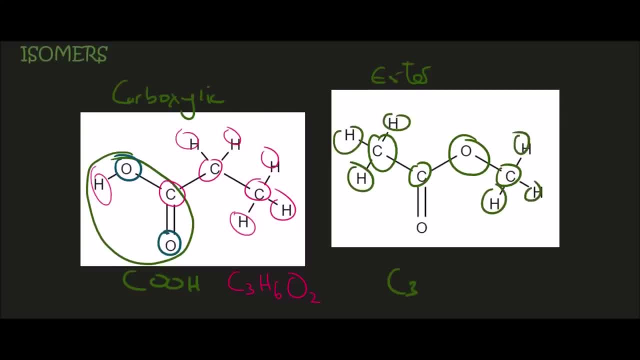 H is one, two, three, four, five, That's C3H6O2.. H is one, two, three, four, five, six, And then oxygen one and two. So once again, these two molecules have the exact same molecular formula. 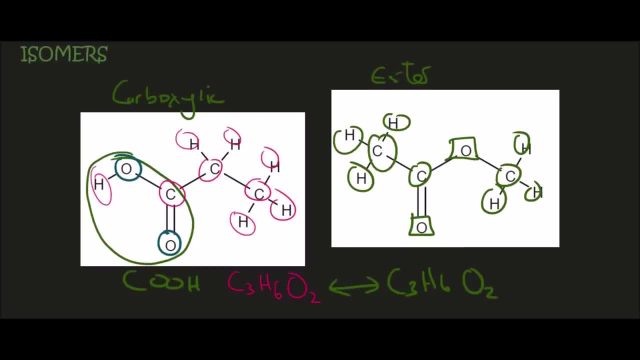 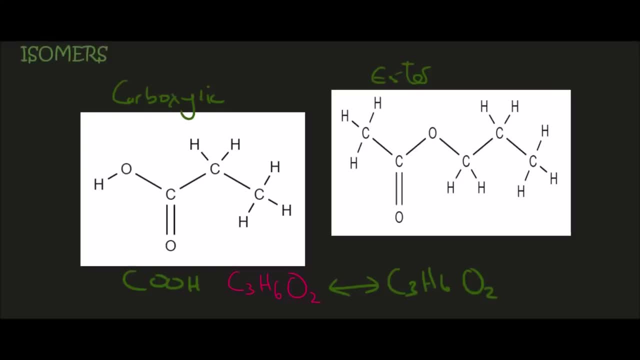 But if you look at their structure, they are completely different. The way that they are arranged is totally different. OK, now, something that we can't do is the following: Here we've got another ester that I've just replaced, But this ester has one, two, three, four, five carbons. 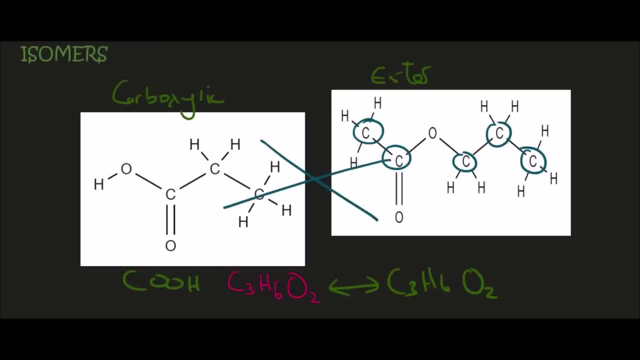 So now we can't compare these two. Obviously we have to have the same number of carbons as our starting point, Otherwise it just won't work. So isomers must have the same molecular formula, But they'll have different structural formulas. 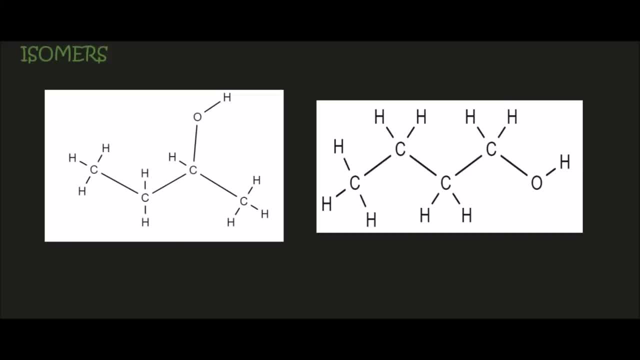 Now things are going to start getting interesting. Why? Because look at these two molecules. The one on the left: what is that? What homologous series is that? Well, it's an alcohol. The one on the right: what homologous series is that? 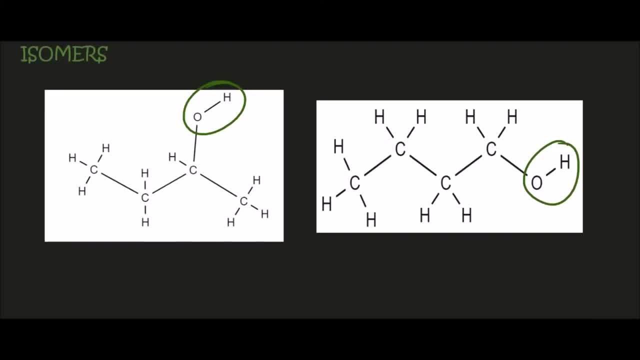 That's also an alcohol, But these two are going to be isomers, Kevin, how is this going to work? OK, Have a look at this guys. So of course, they're going to have the same molecular formula, because the one on the left has one, two, three, four carbons. 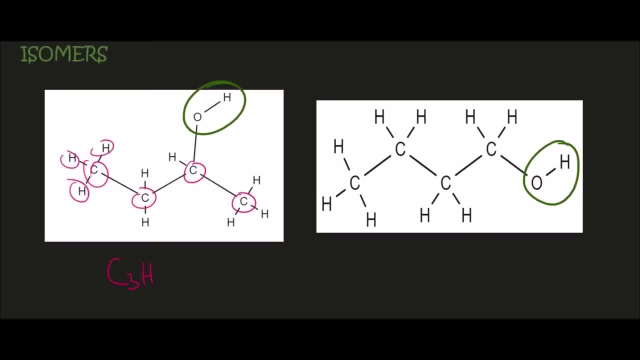 That's C3.. The number of hydrogens is one, two, three, four, five, six, seven, eight, nine. Sorry, there were four carbons, OK, so that's whoops: C4H9.. 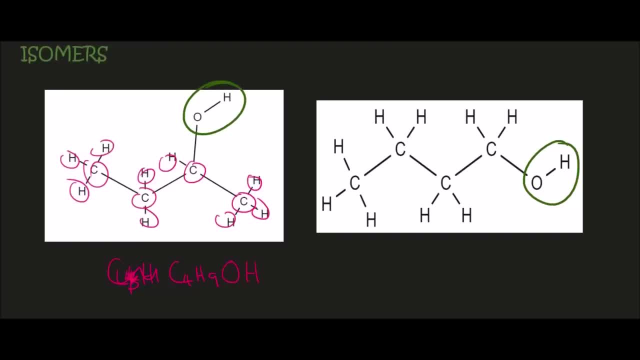 And then there's the OH. Remember, with alcohol you don't count this H over there, You rather write it down. You write it as C4H9, and then you put the OH at the end. We did look at that in one of our previous videos. 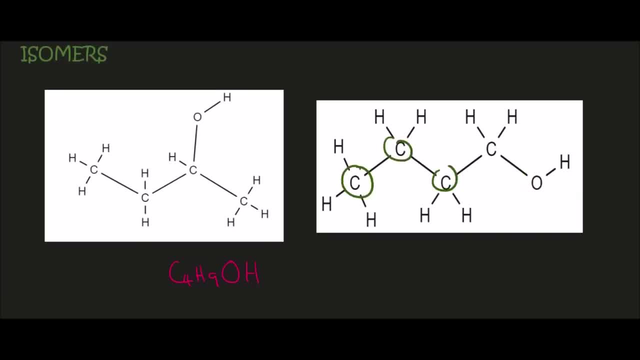 Now the one on the right hand side has one, two, three, four carbons, So C4.. One, two, three, four, five, six, seven, eight, nine hydrogens, And then there's the OH part. 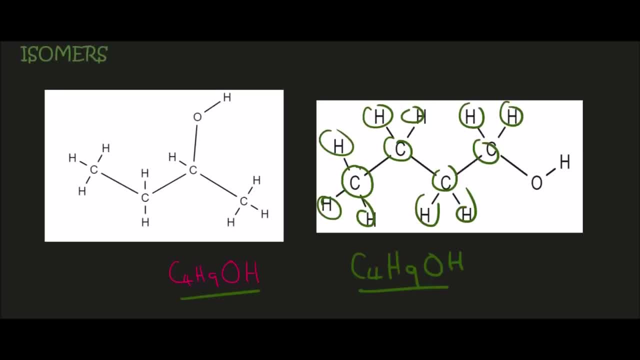 So there we have it. The two chemicals have the same molecular formula. However, the one on the left has its OH attached to a carbon that is somewhere in the middle, whereas this one has an OH attached to the carbon on the end, And so the structure of those two is completely different. 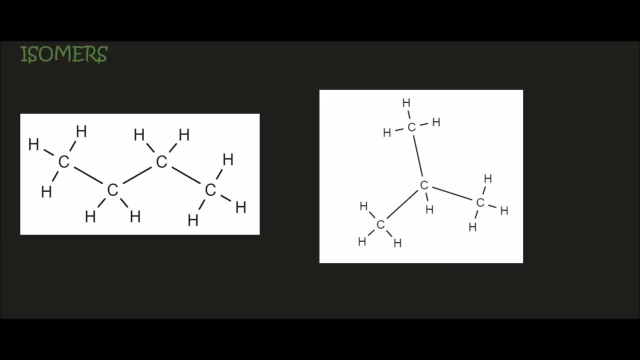 So once again, these are isomers. Now here's our last two that we're going to compare, and then I'm going to summarize. So here we've got alkanes right. We can see on the left and the right they are alkanes. 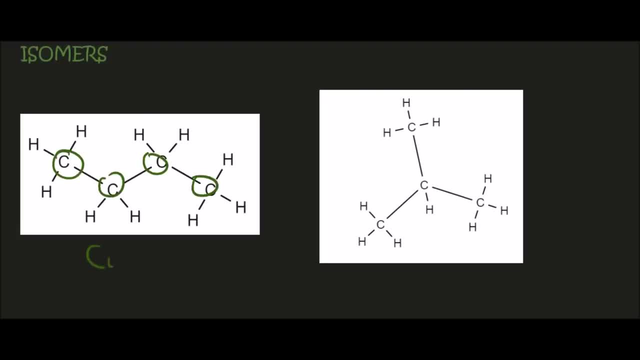 The molecule on the left has one, two, three, four carbons, But the H's there are 10 of them. You can double check me if you want, On the left, on the one on the right hand side has one, two, three, four, five, six. 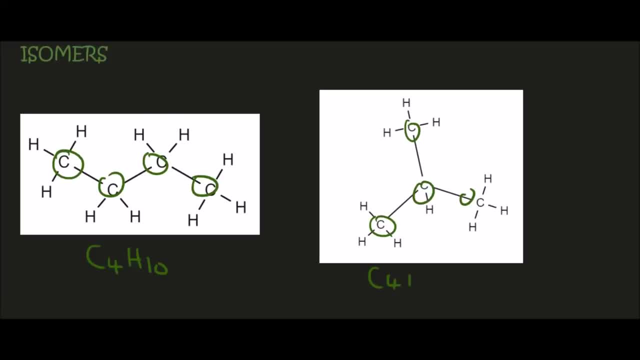 one, two, three, four carbons, And if you looked at the hydrogens, there would be 10.. So these two molecules once again have the same molecular formula, But if you look at the way that they are structured it's totally different. 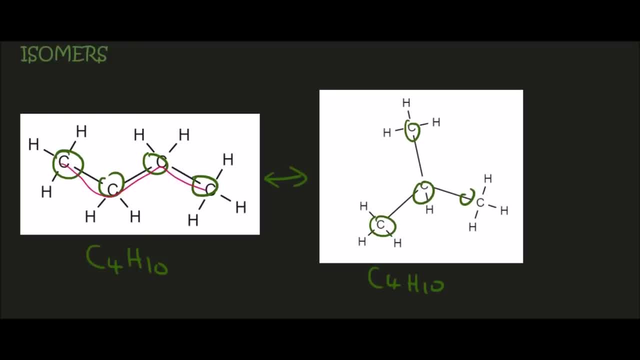 The one on the left has a four chain carbon, or four chain, the continuous chain or the longest chain has four carbons. The one on the right has a three chain carbon. See like that it flows continuously. Okay, If you look at the middle carbon, there's a carb, there's a branch off. that goes like: 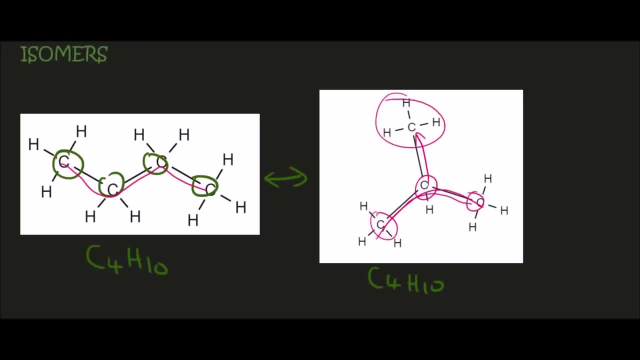 that. I know we haven't dealt with branches and things like that, but we will get to that. But what you must just do now is take my word that these two are also going to be isomers, because they have a totally different structure. 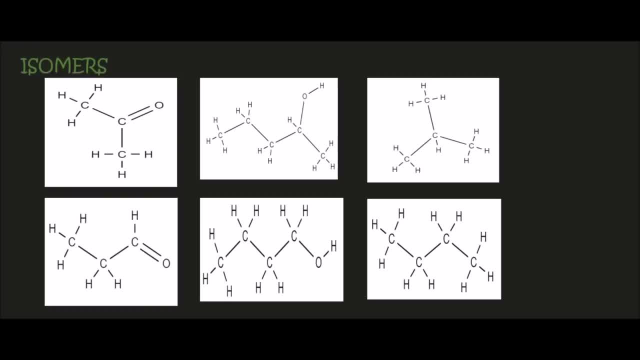 And so, guys, the next minute or two is going to be vital. So we looked at isomers, but now there are three different kinds of isomers and they are functional, positional and chain. So we looked at all three of those in this video, without you even realizing it. 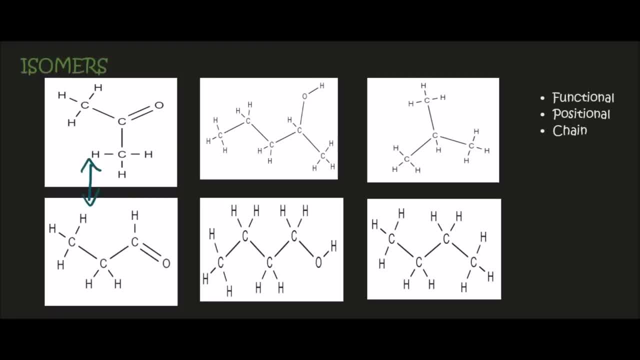 Have a look at the first one. So I'm working in a vertical direction. So this was the aldehyde and the ketone comparison. So is the functional group? remember the functional group is the part of the molecule that makes it do what it does. 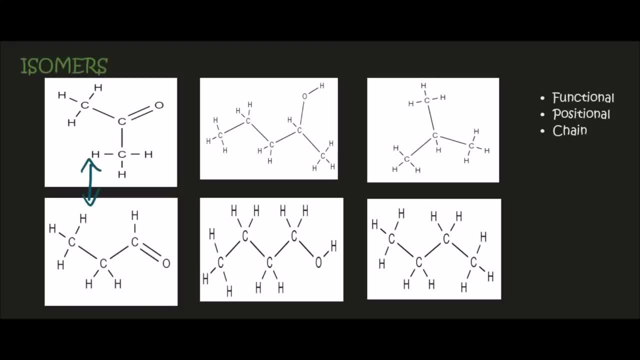 Is that the same for both of them? Well, no, because we said that for a ketone, the functional part is the double bond: oxygen bonded to a carbon that is between two carbons. So remember, we said that it was something Okay. 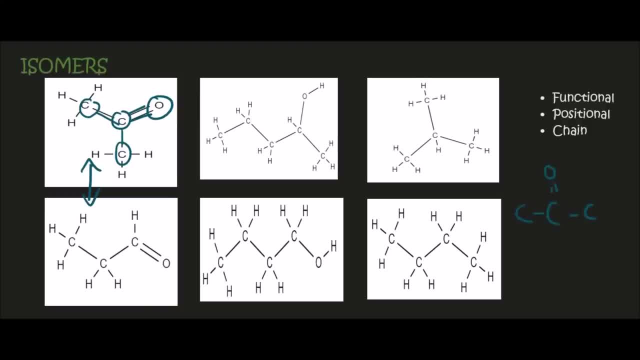 That it was something like this, Whereas for an aldehyde it's just this little piece here at the end, So it's a C double bond oxygen with a hydrogen, So the functional parts are totally different, And so that is called functional isomerism. 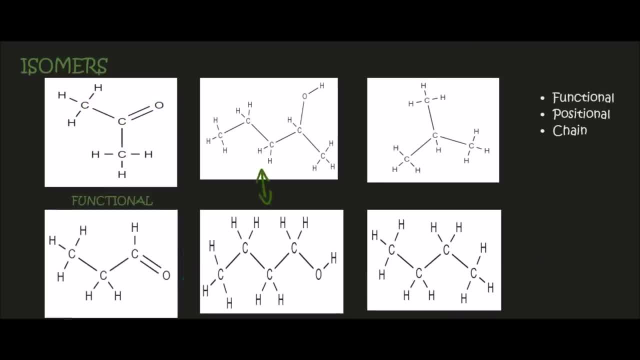 The next ones we're going to look at are going to be these two. So we looked at these and we saw that this one was an alcohol and so was this. They have the same number of carbon, same number of hydrogen. Everything is the same. 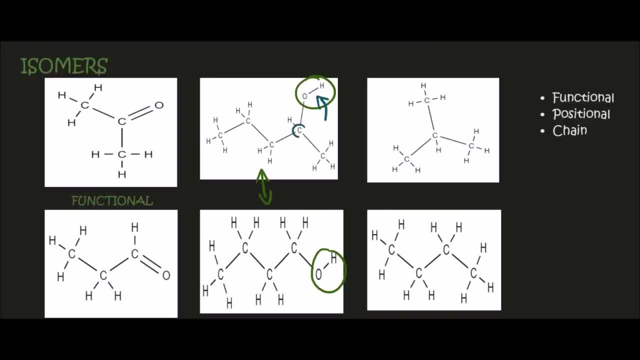 However, This Is On one of the carbons in the middle of the chain, whereas this OH is on one of the carbons at the end. So they are both going to be called alcohols, but they are still considered to be structurally. 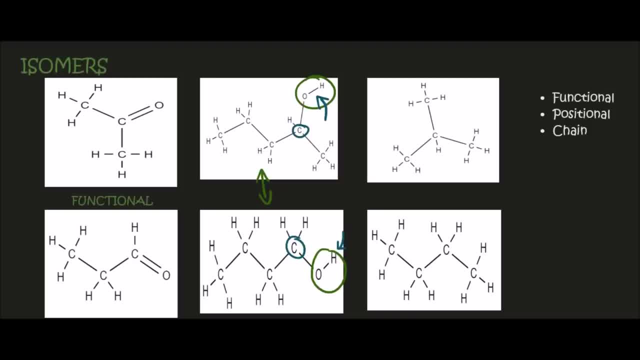 different. So they are both alcohols, so it's not going to be functional. Their functional part is the same, so they're not functionally different. Their main chain: if you look at their main chain, there is one, two, three, four carbons. 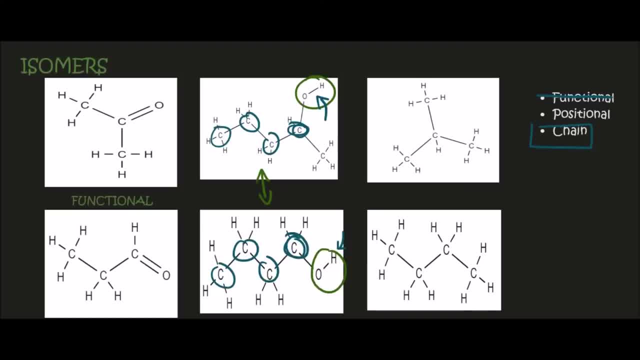 in that one. So the main chain is the same, And so it's the position of the functional part, which is this part. here That position is different. If we label this structure on the right, from right to left, that would be carbon number. 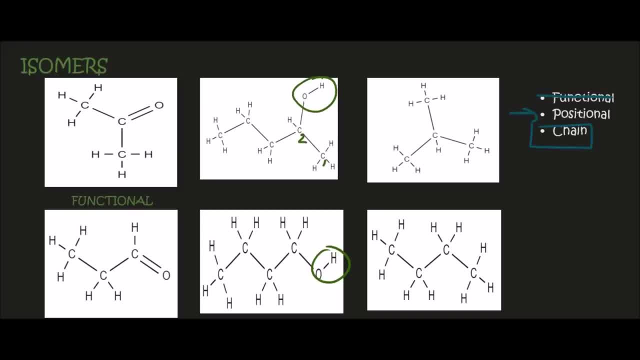 one, and that would be carbon number two. So we can see that the OH is on carbon number two. If we look at the one at the bottom, the OH is on carbon number one. So the position of the functional part has changed. 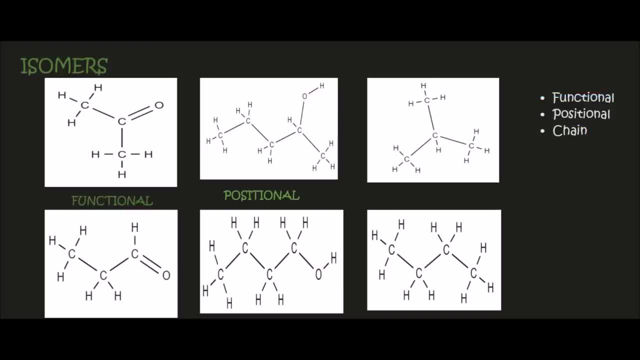 And so that is called position, That is called positional isomerism. And then, with the last one, we know that both of these are alkanes. How do we know that? There's just carbon hydrogen single bonds wherever we look? 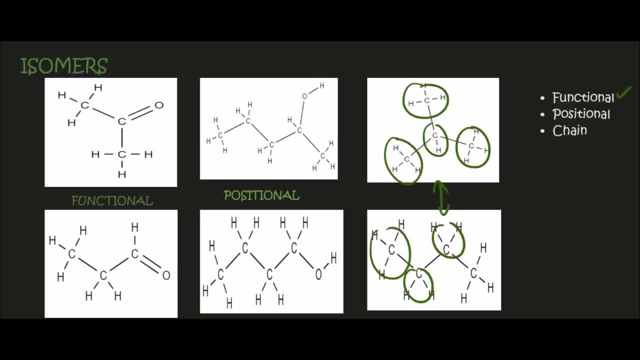 So the functional part of both of those is the same. It's an alkane, The position. we can't really look at that, because I mean the position, the functional group for an alkane. remember, it's all the single bonds.